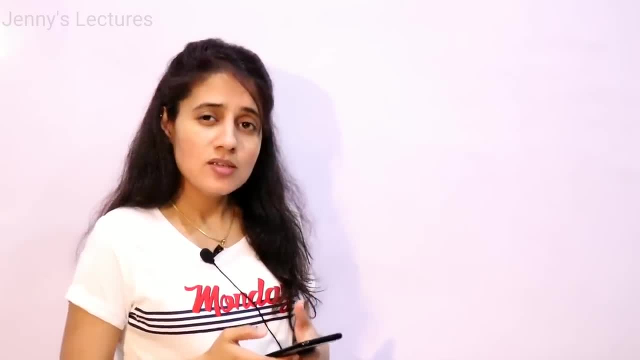 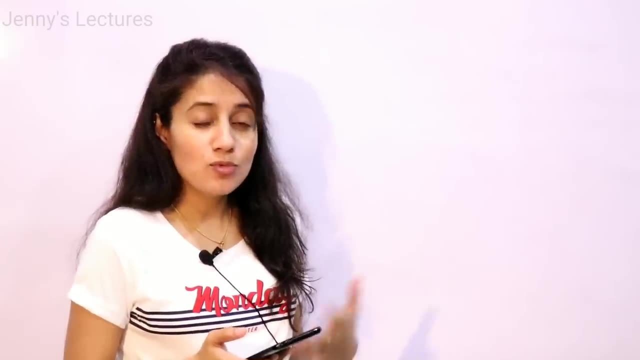 likes came, so many dislikes came. It's not like this that something happens in monetization or something like that, But still, when you get likes then you get a motivation And when you get dislikes then it feels like. I guess you guys understand me. 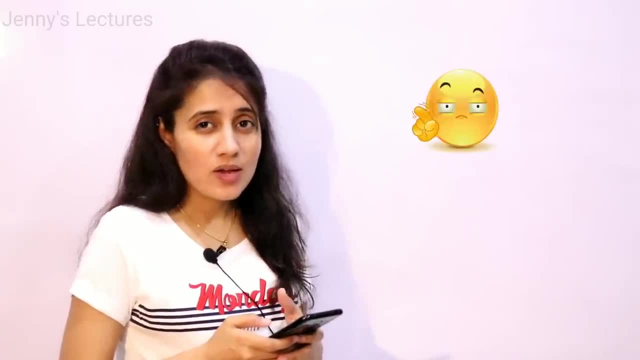 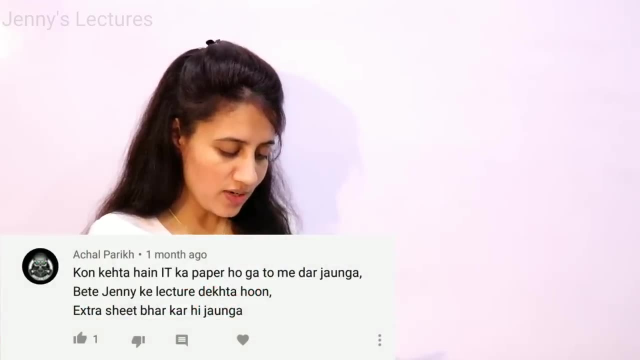 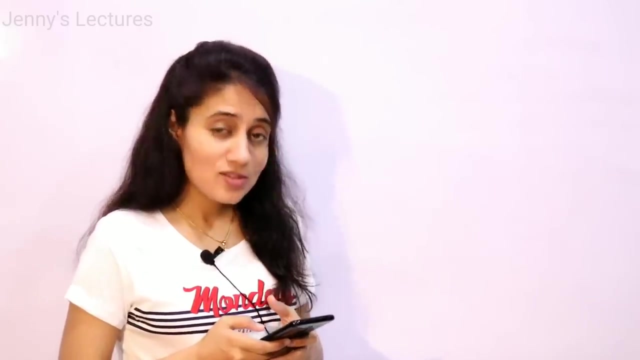 I don't understand whatever I am teaching, So please don't dislike. Who says, if the IT paper is done, I will get scared. I will watch Jenny's lecture. I will fill the extra sheet. Wow, Leave it for someone else. 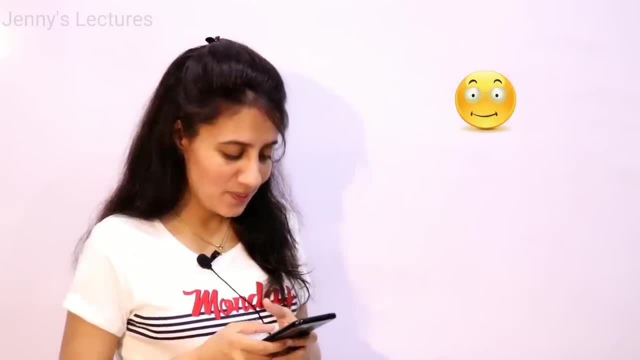 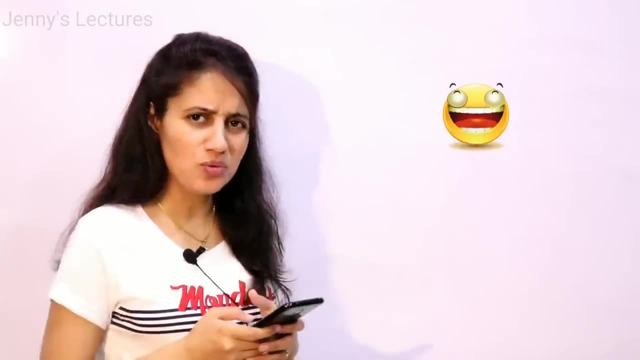 too. Sometimes fill all the sheets yourself. Well, all the best. Do you go to doctor's gym? in Kolhapur I saw someone similar looking to you. No, never Do I look like that as soon as I go to the gym. 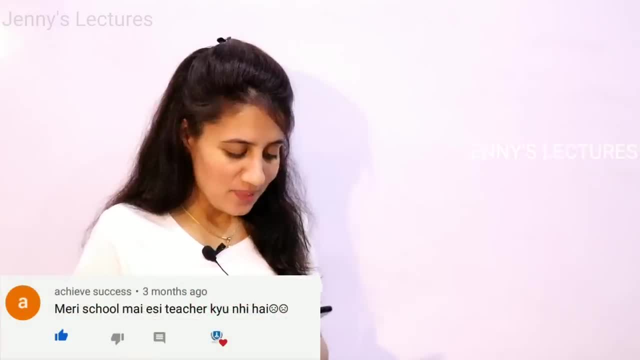 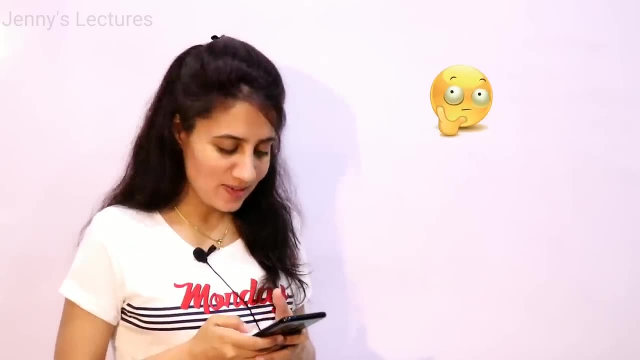 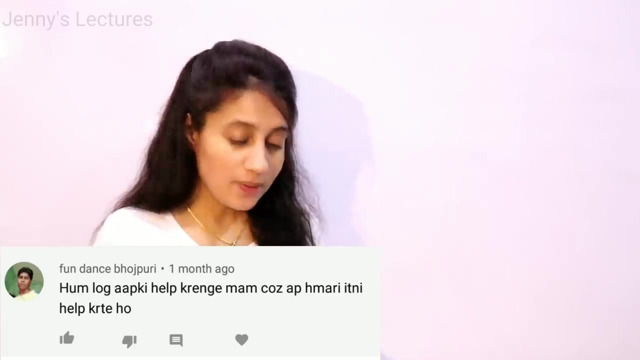 No, Why isn't there any such teacher in my school, In the school Dear? what kind of teacher do you want? We will help you, ma'am, because you help us so much. Well, thank you, But how will you help me? You are going to do one thing: If you feel that my videos 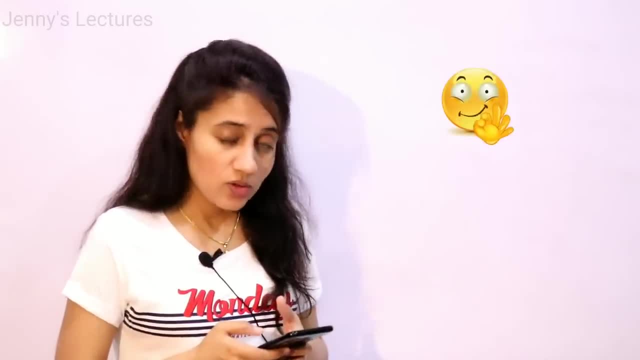 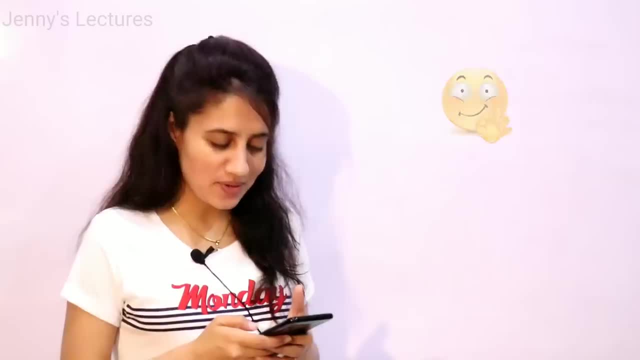 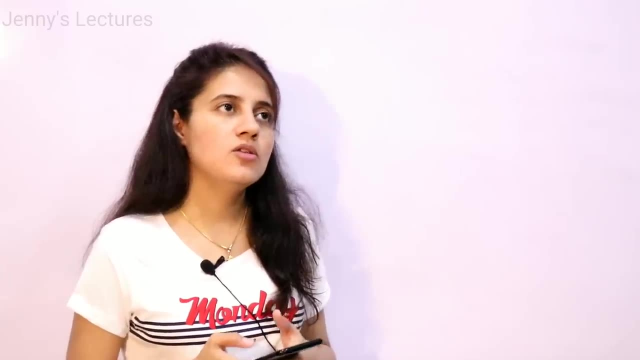 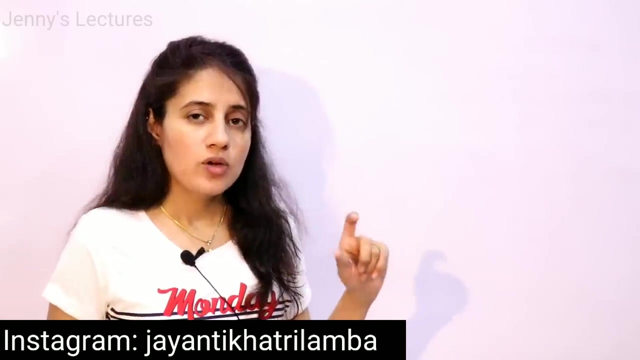 leagues or your juniors. right, that is enough for me. thank you, ma'am. vlog channel ka link de. do see my vlog channel. you can get everything about my vlog channel on my instagram, right that is? the handler is jayanti khatri lamba. so i have recently uploaded one new video on that vlogging channel. 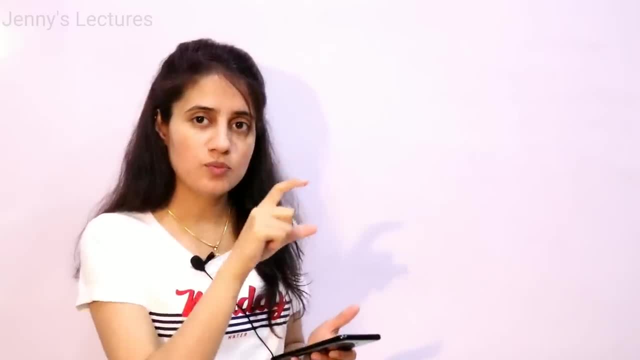 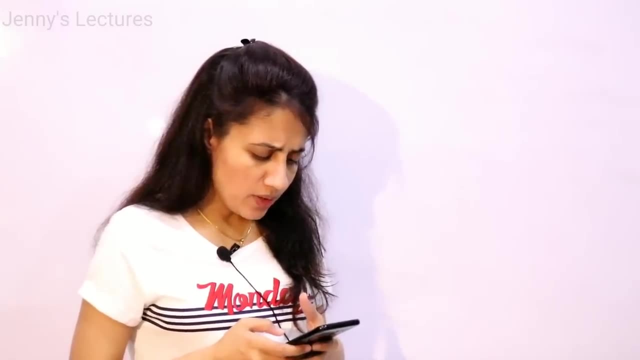 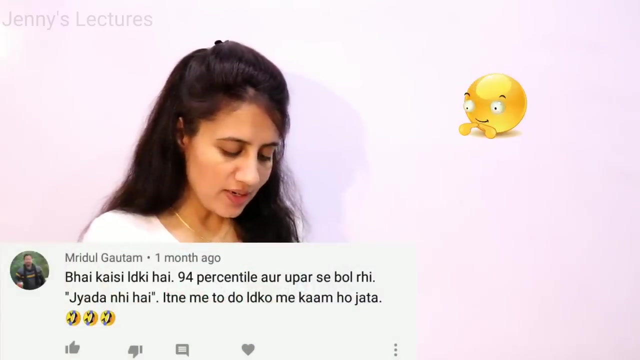 you can go to my instagram and in their bio profile bio you will get a link so you can go to vlog channel through that. i am from nepal and i pay a fee at college, but i learn from you. thank you, dear bhai. kaisi ladki hai 94 percentile aur upar se bol rahi jada nahi hai. 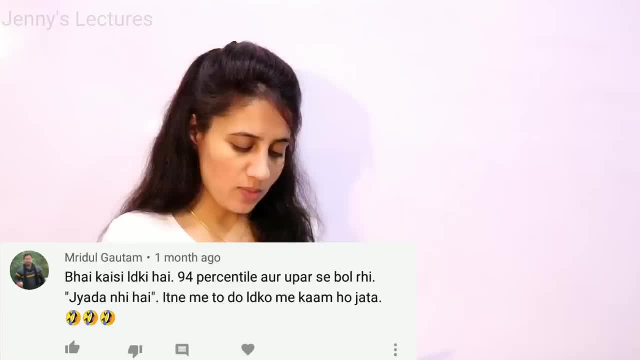 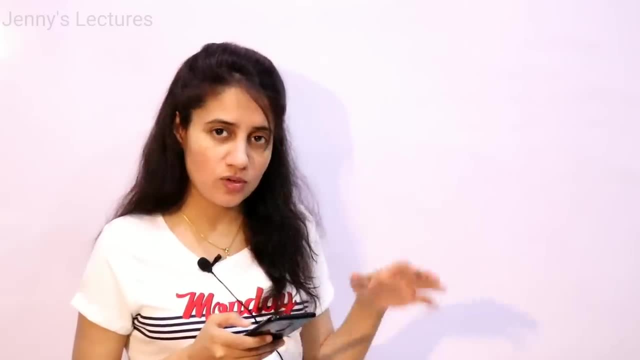 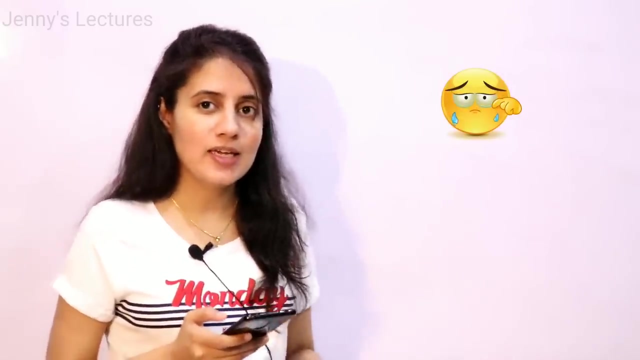 itne mein do ladko mein kaam ho jata. yeah, yeh comment hai shayad mera that i was telling my gait score around. it was around 92- 94 percentile. you actually i was expecting around 98 or 99 to get into iit, but 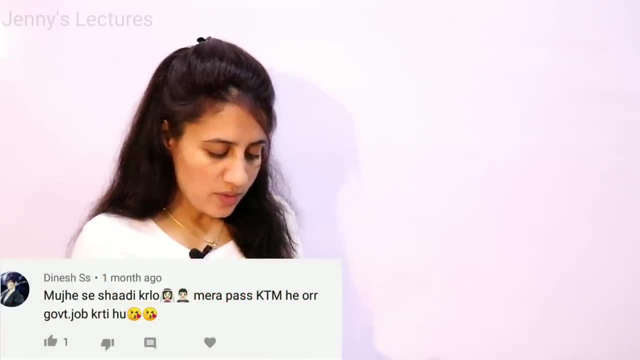 woh nahi mila. that's why mujh se shadi, karlo, mere pass ktm hai achha, aur government job karti hoon. i am sorry, i am straight. by the way, your name is dinesh and you said government job karti hoon. 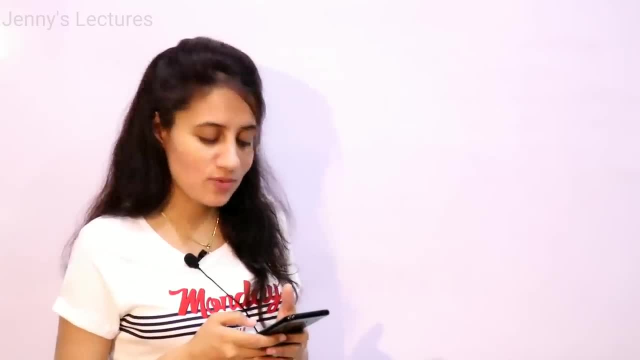 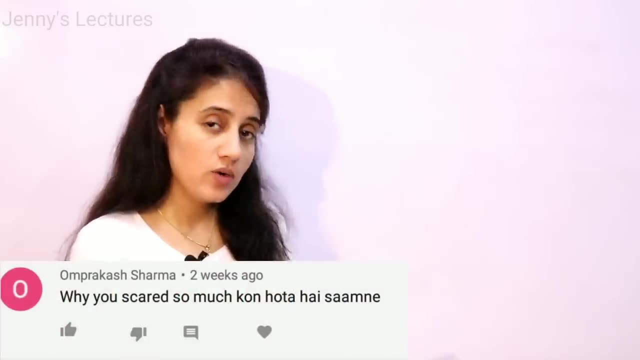 agar karti hoon, toh waise bhi main nahi kar sakte. aapke paas chai kuch bhi hoon. i am sorry why u scared so much? khon hota hai samne. anyone ask me kyun darthe hoon? 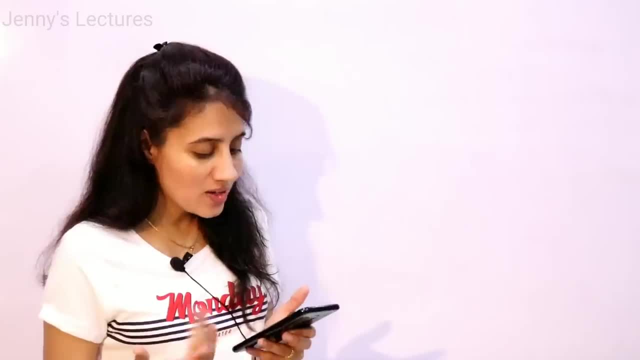 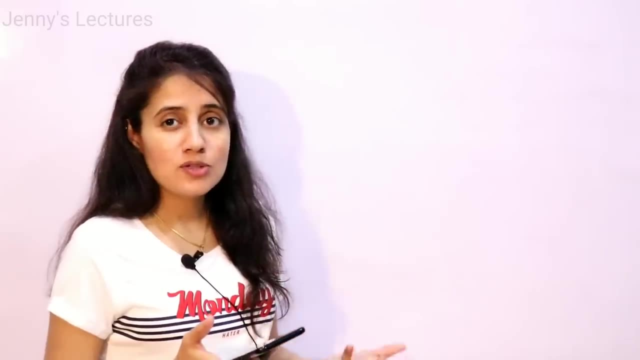 actually you guys are in front of me. i am assuming you all are sitting in front of me. asaa feel hota hai pata niy ab launga samjh aari hai not how you make comment. okay, you have, were waiting. Minecraft create these on your China, I guess, which handle your tomb利. 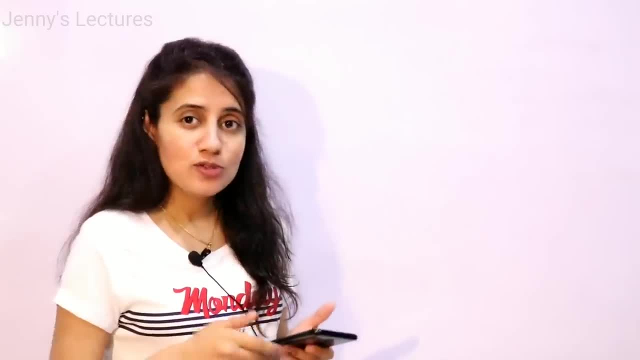 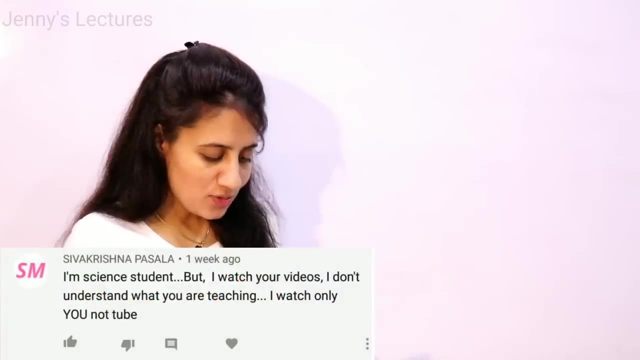 he. its very tough create videos on YouTube channel. I get what Kindr YouTube video bhai recently Adit. probably I am going to end of my life why you scared mindful piece, sister. I am science student but I watch your videos. I don't understand what you are teaching. I watch only you, not tube. 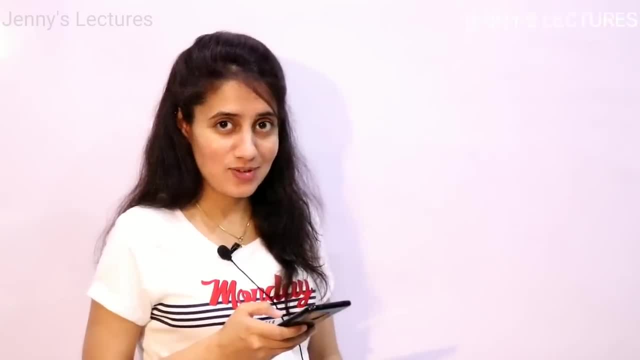 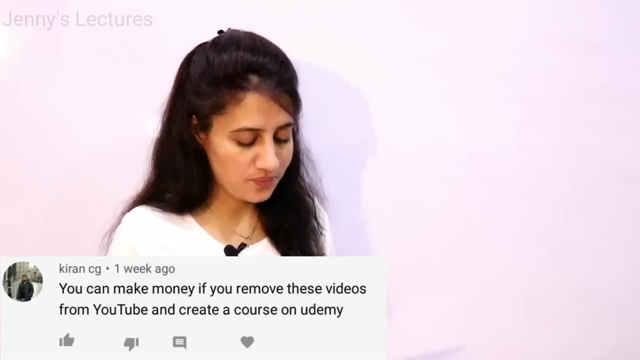 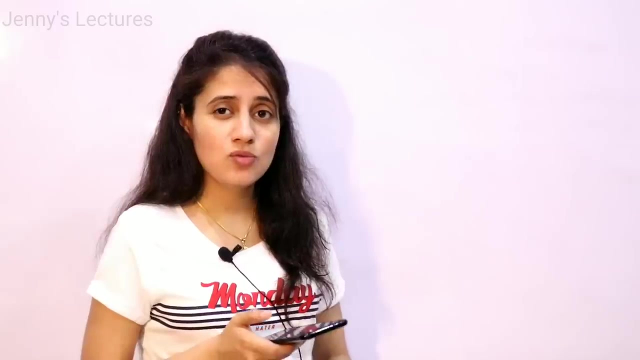 Don't waste your time. invest your time. okay, You can make money if you remove these videos from YouTube and create a course on Udemy. Yeah, I can do that, But actually I feel that many students- I know many students- are there who are not able to. 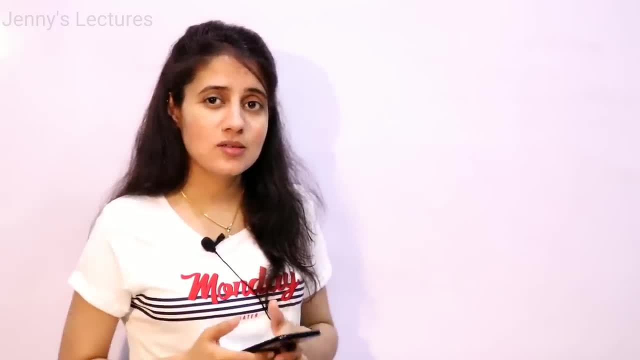 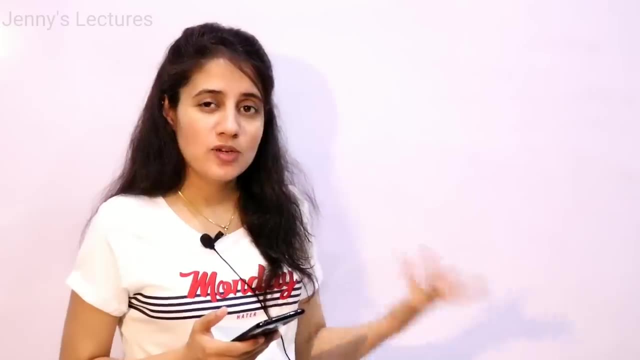 pay. This is to be very honest with you guys. what time, say my sociality, could say: you know, social carnega, Yeah, which is a but you will put on a car. You're very but. you're there, but unfortunately, because of some circumstances, as a honey pie. 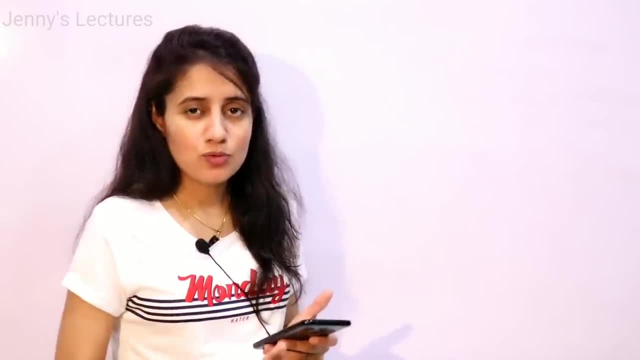 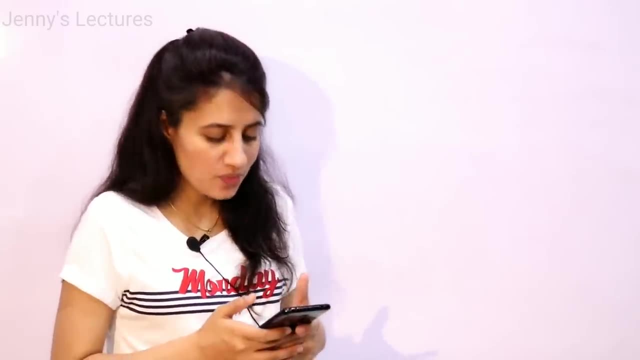 So I be a platform Mila. Hey, YouTube kid through so much. I think you may free of cost job in knowledge. Maybe I'm a pro white girl. Guys, subscribe her. what you are waiting for? She helped a lot. Thanks, They well. thank you. 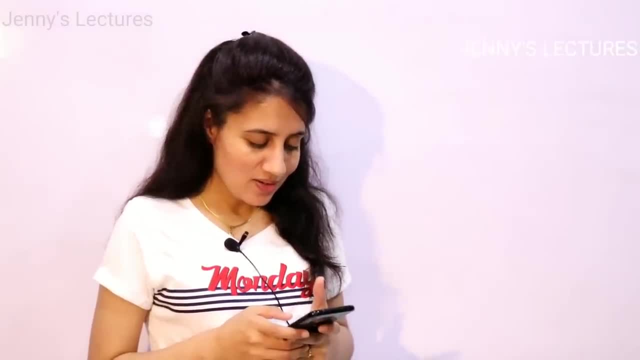 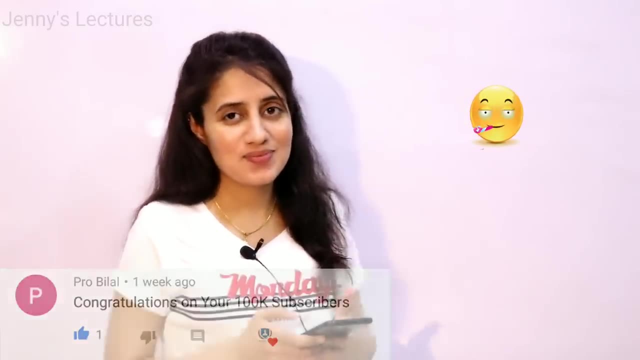 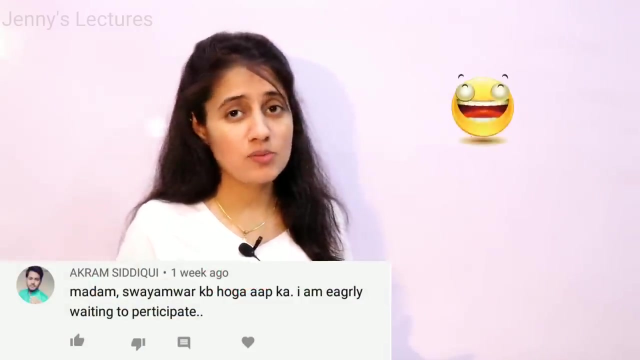 Subscribe group. they carry, Bobby. Congratulation on your 100k subscribers. Yeah, Now we are a family of 100k subscribers. Thank you, Madam swamber. cup hookup. I'm eagerly waiting to participate. Oh dear, I'm so sorry You're late. 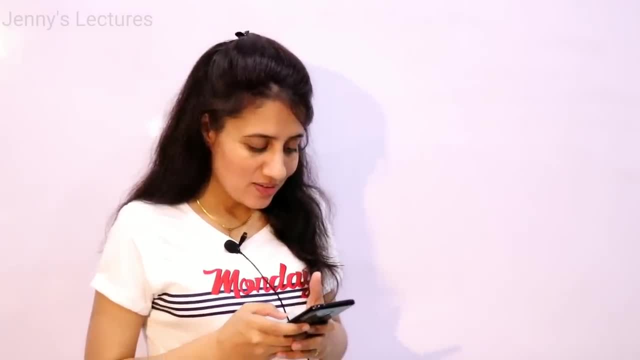 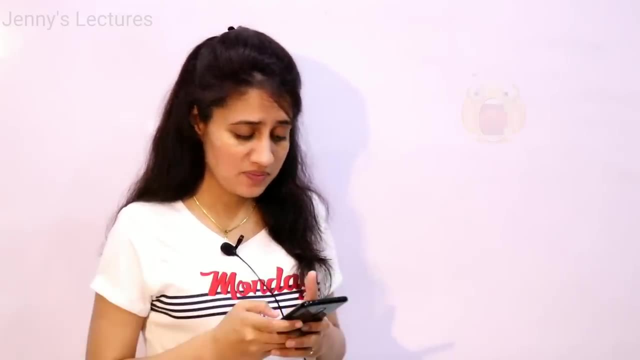 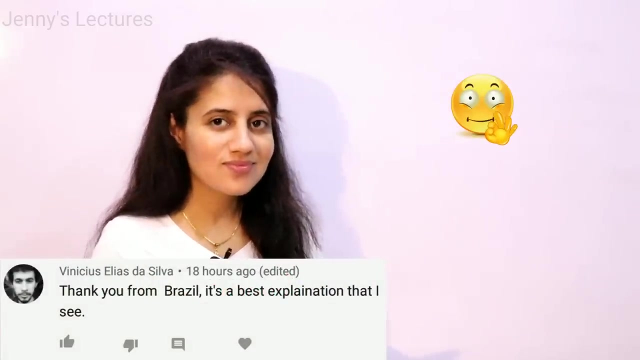 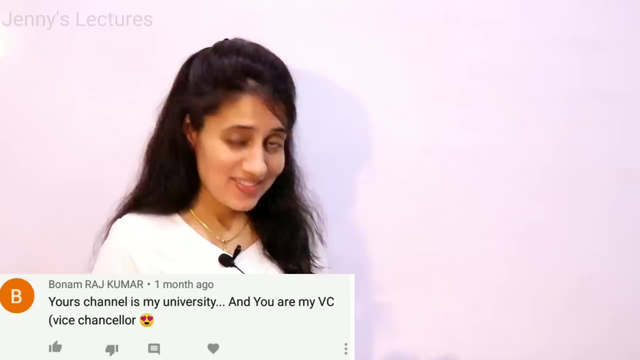 What the ho Guerrilla There up me. I didn't what the cya Really. Yes it. Thank you from Brazil. It's the best explanation that I see. Thank you, dear. Your channel is my university and your my VC. That's a great Compliment for me, Thank you. 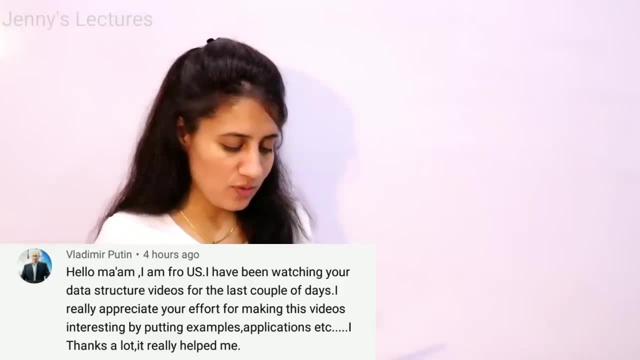 hello, ma'am. i'm from us. i have what. i've been watching your data sector videos for the last couple of days. i really appreciate your efforts for making these videos interesting. interesting by putting examples, applications etc. i thanks a lot. it helped vladimir putin, you sure you are. 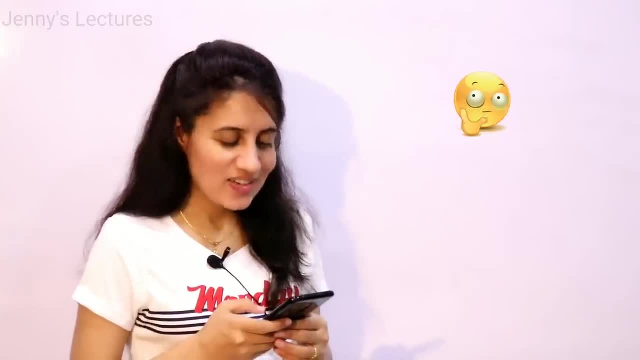 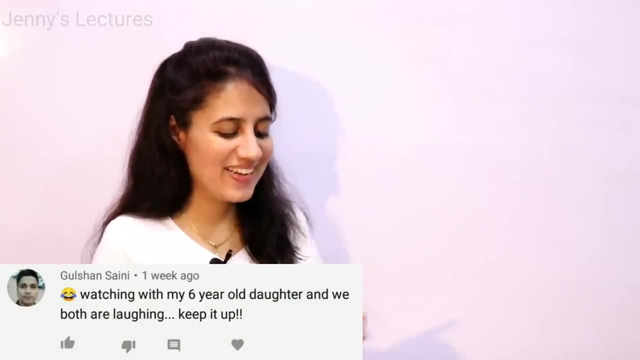 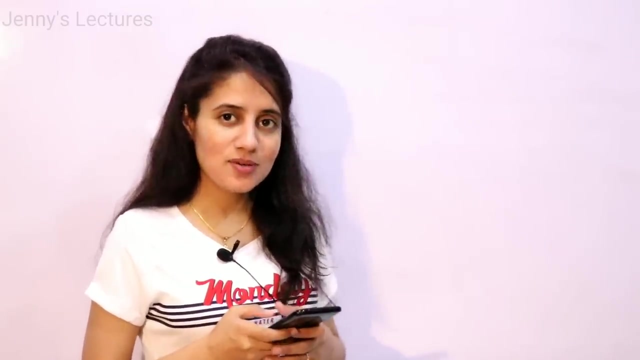 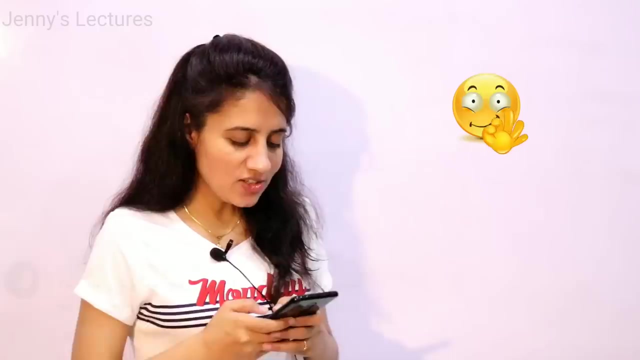 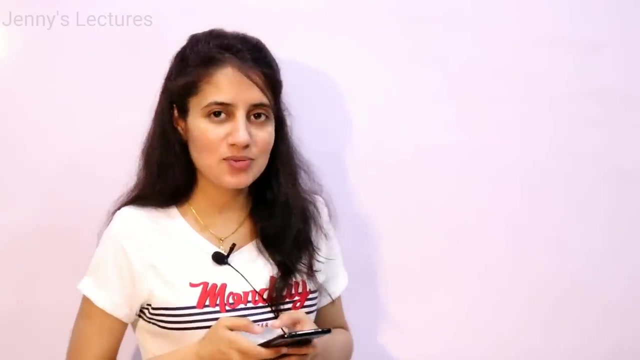 from us, not from russia. well, thanks, vladimir. watching with my six-year-old daughter and we both are laughing. keep it up. great. well, love from my side for your daughter. teachers like you are needed seriously, who gave not only theories and codes, but knowledge also. thanks, anuma. i'm always happy to share the knowledge i have. 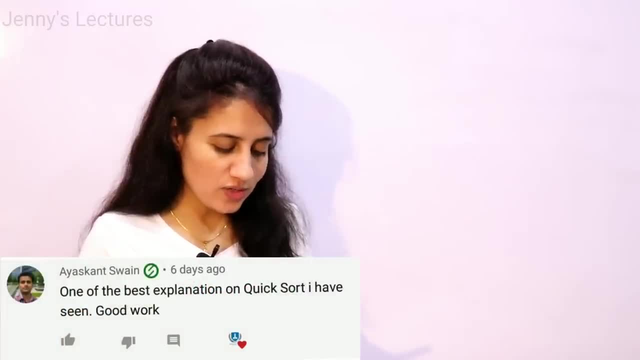 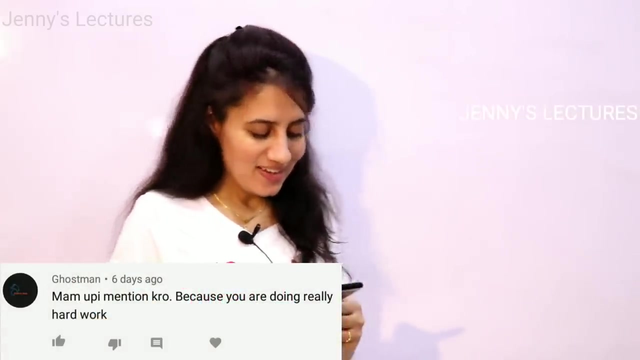 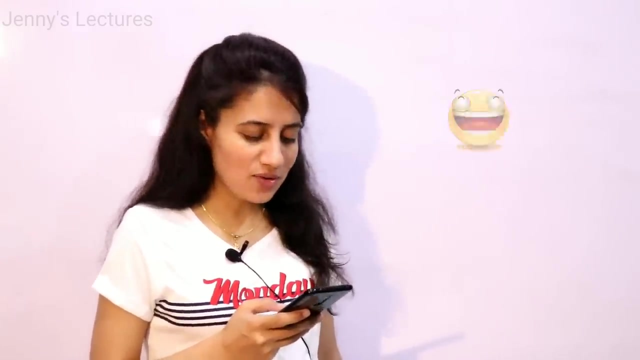 one of the best explanation on quicksort i have seen. good work, thank you. oh, you have that badge in front of your name means you have joined my channel. ma'am upi mentioned crow because you are doing really hard work well, thank you for your concern, dear, but your comments, your love, your support is enough. 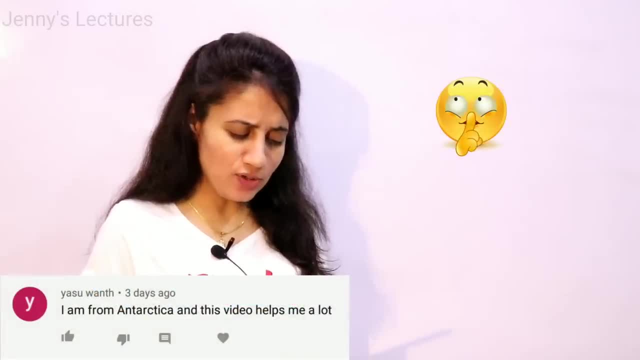 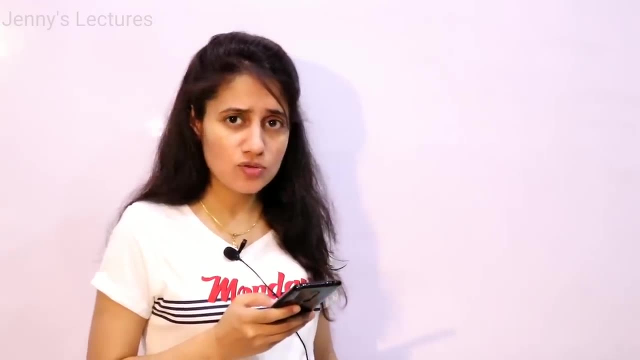 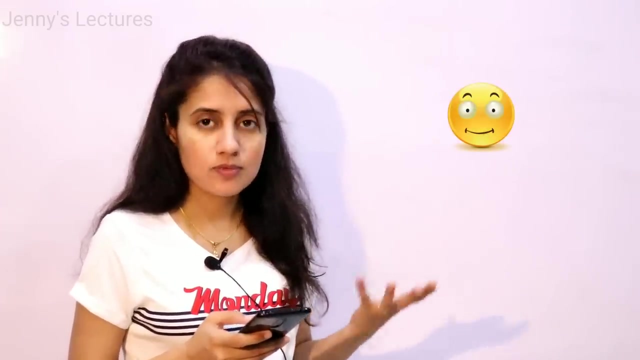 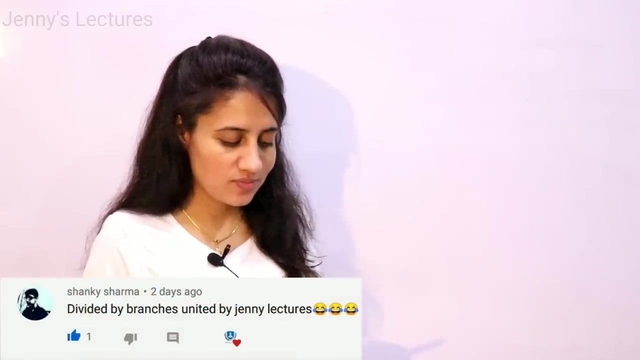 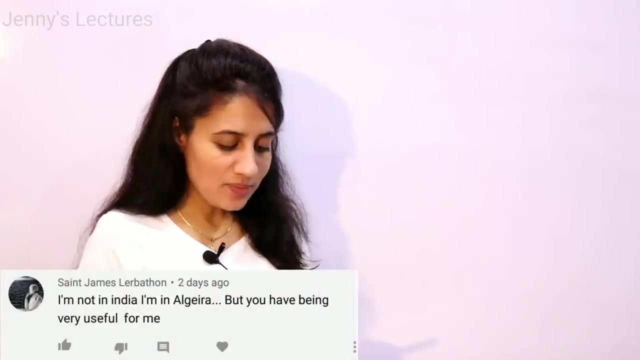 for me. i'm from antarctica and this video helps me a lot. and also i wanted to say that i'm from india and i'm from latin america, seriously, because i guess no one lives there now. i'm expecting a comment from someone that, ma'am, i'm from mars and i'm watching your videos. divided by branches, united by jenny lectures. you're definitely from, not from cs or it branch, right, i'm not in india, i'm algeria, but you have been very useful for me. thank you, dear thanks from india. 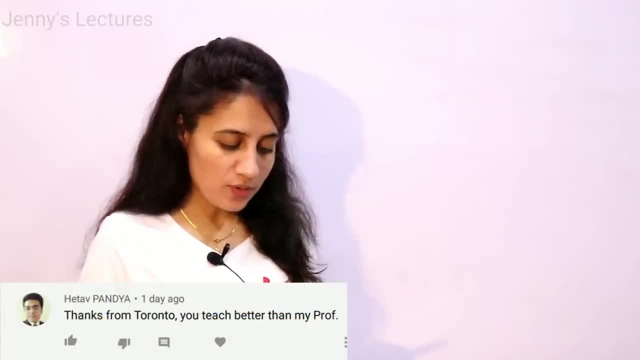 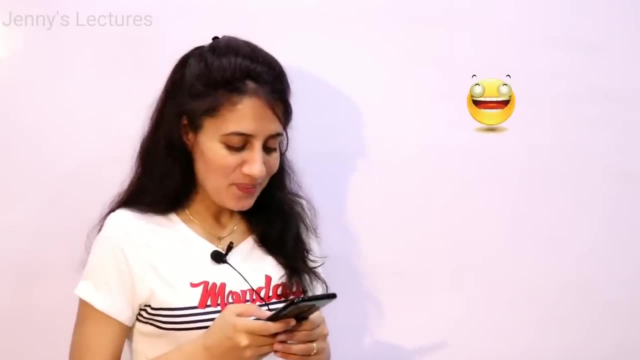 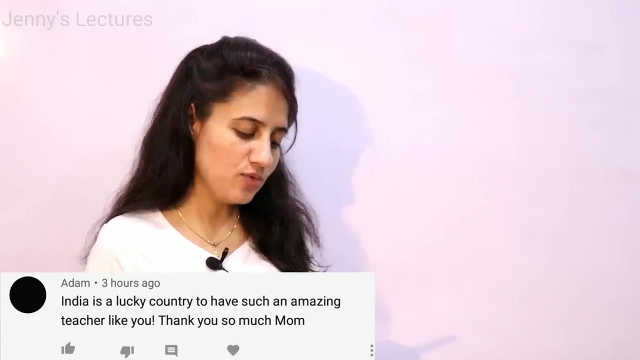 thanks from toronto. you teach better than my professor bohot international fan following ho rahi hai meri thanks, dear india is a lucky country to have such an amazing teacher like you. thank you so much. well, thank you. well, i guess i am lucky to be born in india. 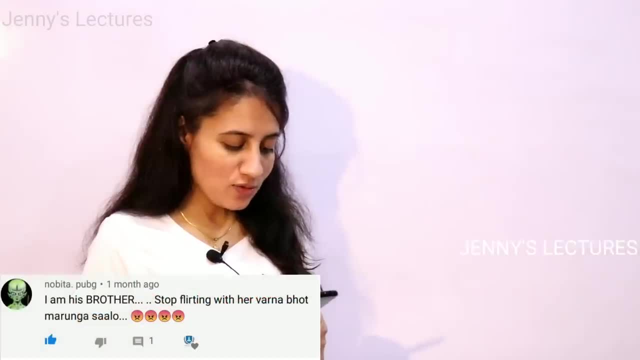 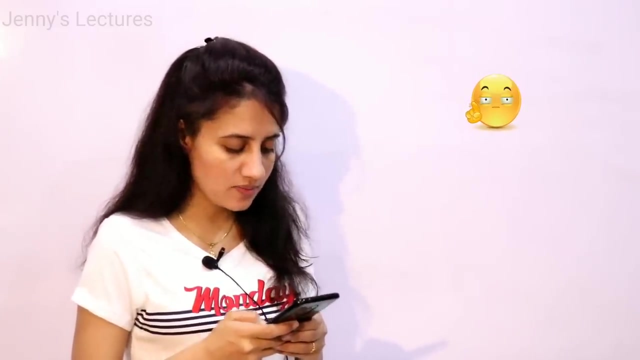 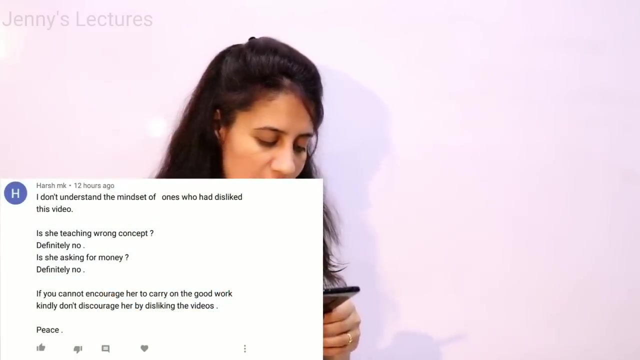 i am his brother. stop flirting with her. vanna bohot marunga nobita dot pubg. you see, in my family i have nobita and pubg dhyan rathna. it's a lengthy one, but i really like this comment. i don't understand the mindset of the ones who had disliked this video. 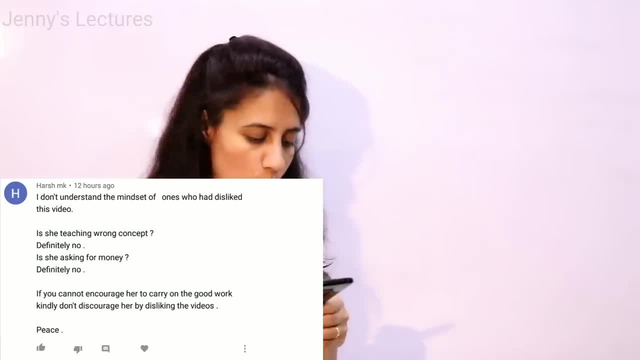 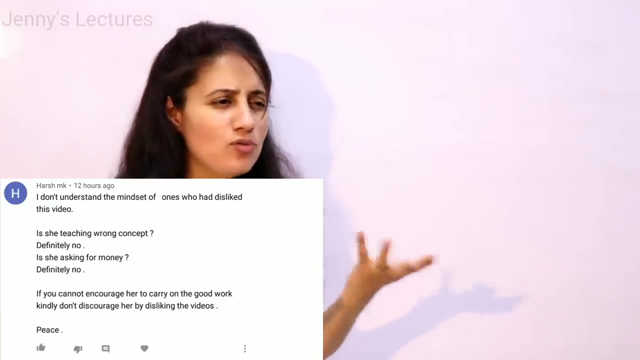 is she teaching wrong concept? no. is she asking for money? definitely no. if you can't encourage her to carry on the good work concept, kindly don't discourage her by disliking the video's piece. well, that's exactly i want to say, because, yeah, around one or two percent comments i am getting. 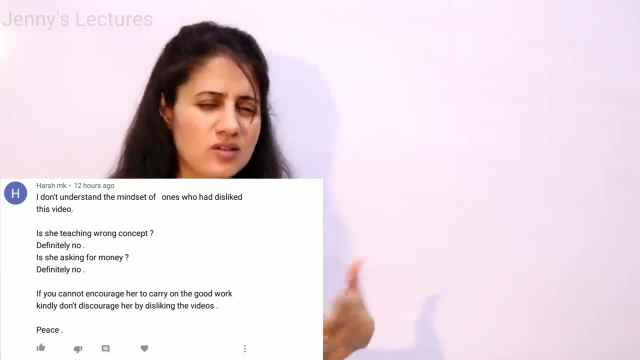 those who use abusing words also and these kind of comments, some discouraging comments and hate speech and all. but yeah, i am not teaching any wrong concept and definitely i am not asking for money. you are not paying anything to me, right? so i guess if you cannot like my videos, then i will not do it. 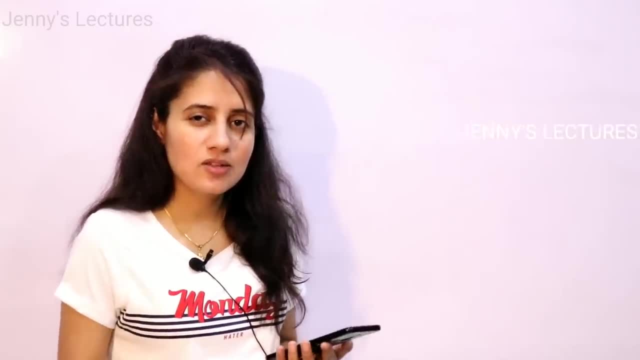 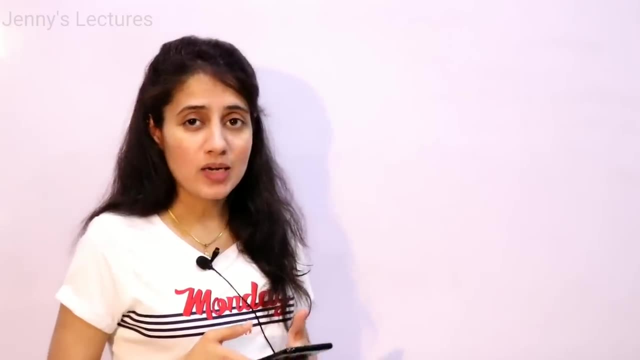 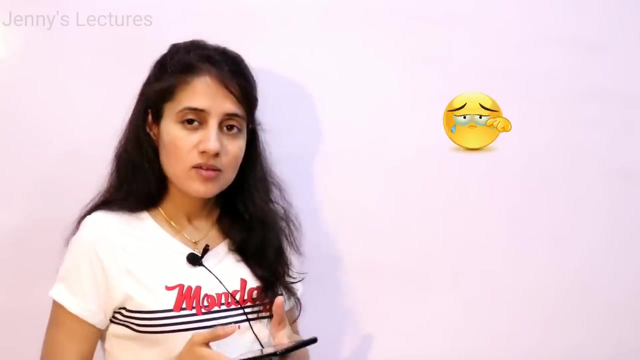 so i guess if you cannot like my videos, then i will not do it. if you can't like my videos or you can't make good comments, then its better you don't do any comment. you not know how much hard working people are for В Defense to make your videos and to teach you.